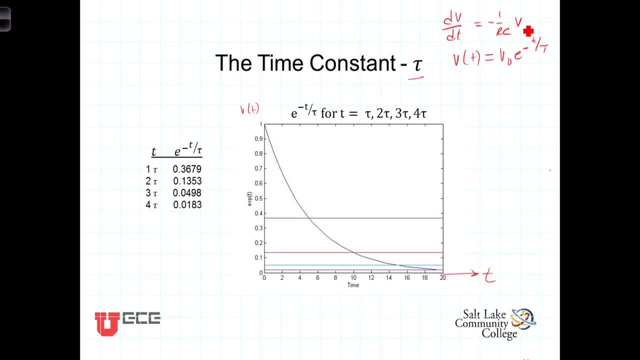 What this differential relationship is saying is that the larger V is, the more rapidly it's changing, and the more it's changing, the more it's changing. So that's the differential equation that describes it, And the change, in this case because of the minus sign, is that it is decreasing. 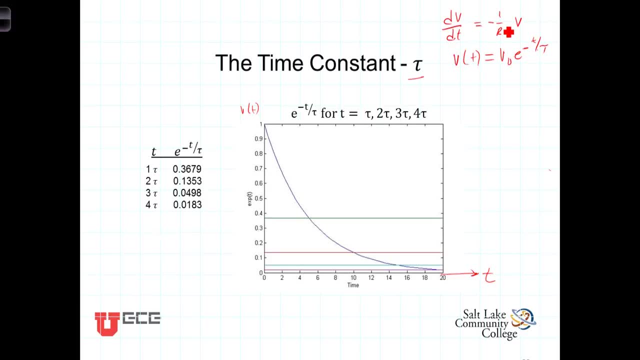 The derivative is negative. So for large V we'll have a large and decreasing voltage. The slope, which is the derivative at the point, is negative and it's relatively large. As V gets smaller, the derivative continues to be negative but becomes less and less. 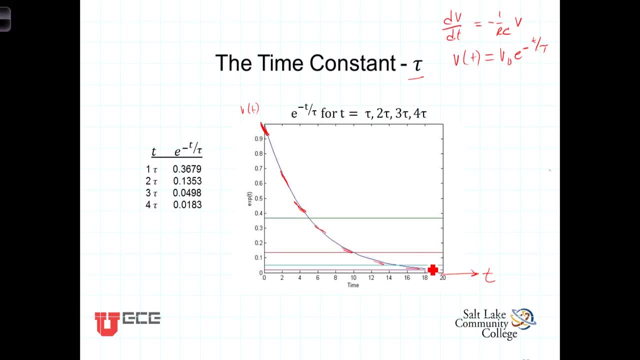 The slope is becoming less and less as V gets smaller. So in fact, as we knew it had to, this relationship here, or this expression, satisfies graphically also our understanding of what this differential expression is describing. Now let's look at the effect of this value tau. 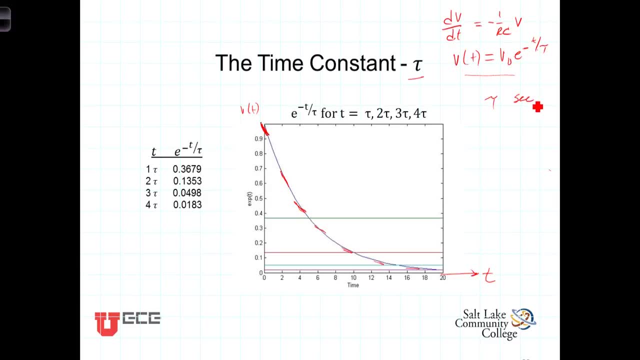 It's the time constant Tau has the units of seconds. It's a measure of how quickly the circuit responds. To understand that, let's evaluate e to the minus t over tau. for values of t equaling 1 tau, 2 tau, 3 tau and 4 tau, 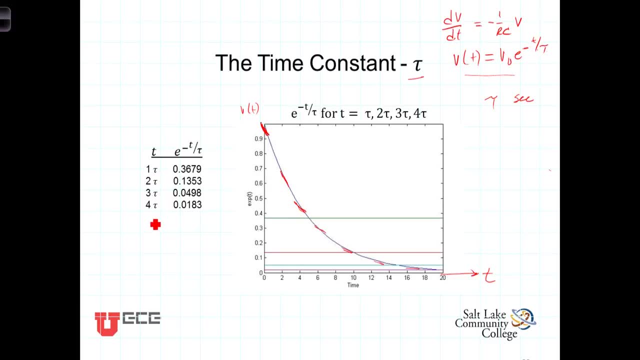 So at t equals tau, we will have e to the minus tau over tau, That's e to the minus 1.. If you get out your calculator, you'll see that e to the minus 1 is approximately. well, it's equal to this, which is approximately 0.37.. 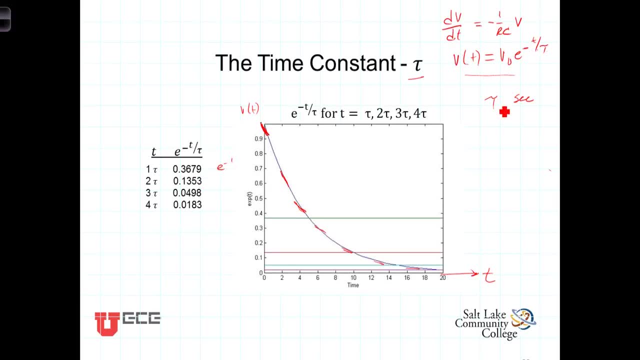 So our function up here, V at 1 tau, is approximately equal to- again, we're going to round that off- to 0.37, 0.37 V naught. So within one time constant, there's 0.37.. 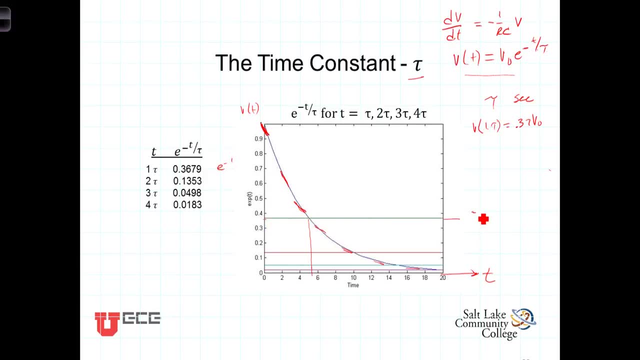 That line there corresponds to a tau or t, rather equaling 1 tau. Now the value of the voltage across the capacitor has decayed down to only 37% of its original value. or to put it another way, in the first, one time constant this circuit. 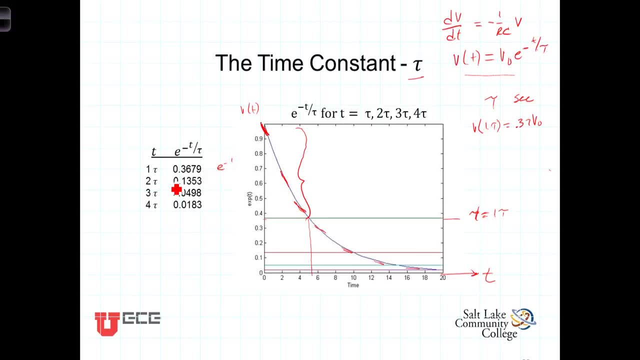 has lost. what is that? 93, or no 63,? it's lost 63% of its original value. or we could also say, in the case of a circuit, it's lost 63% of its original value. 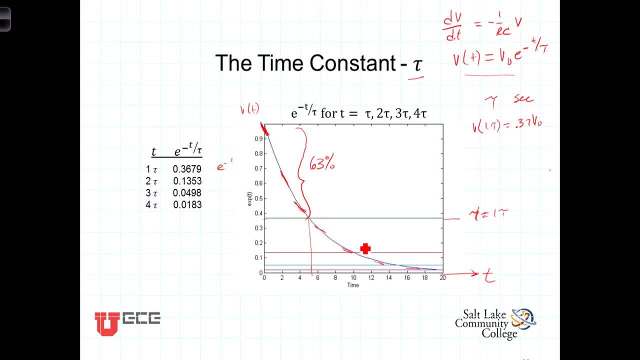 In the case of the step response, that we have gone 63% of the distance to our final value. Now let t equal 2 tau, E to the minus 2, tau over tau is e to the minus 2.. Get out your calculators again. and e to the minus 2 is approximately equal to 0.1353,. 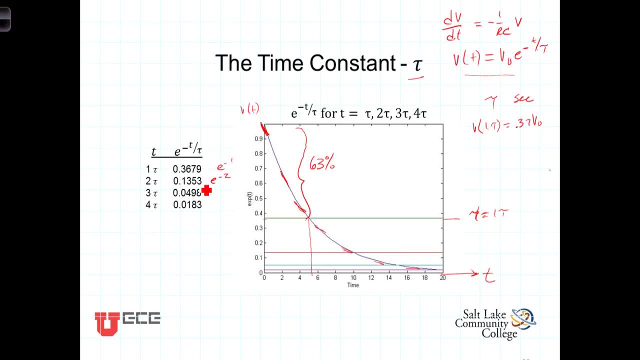 or let's round that off to 0.14.. So at t equals 2 tau, V of 2 tau will equal again 0.37.. That's e to the minus 2.. Again, just rounding out to about 0.14 V naught. 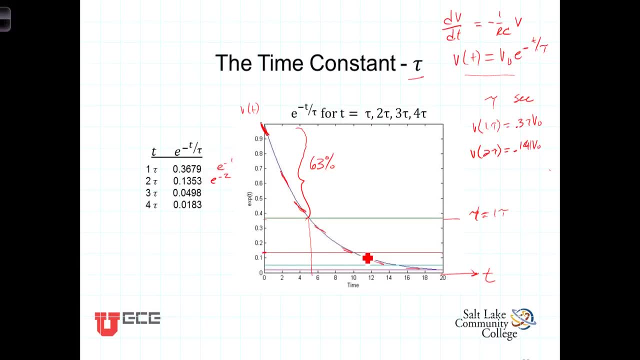 This line. here it's about 0.14.. That corresponds to t equaling 2 tau. At 2 tau, then we have dropped down to only 14% of our original value, or we've then dropped 86%. 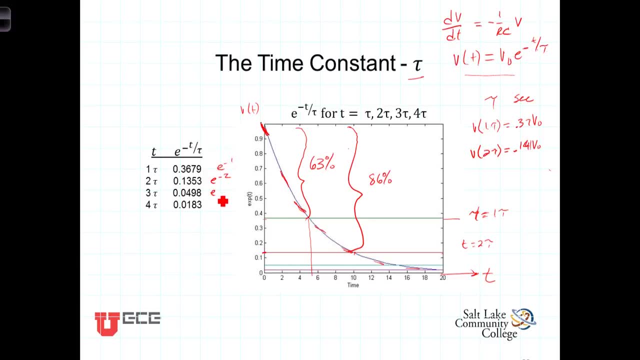 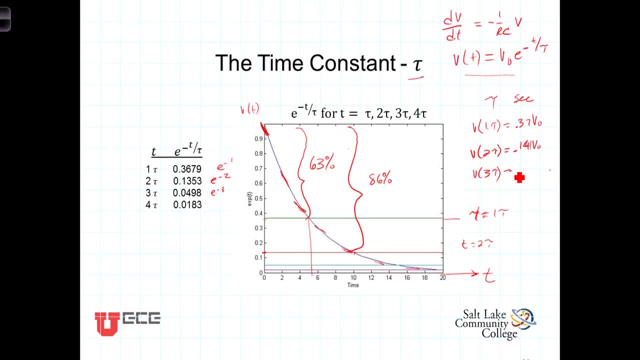 V of 3 tau is approximately equal to 0.05, or 5% of its original value, which means that we've gone 95% of the way to our final within 3 time constants. Finally, t equals 4 tau. we'll have e to the minus 4.. 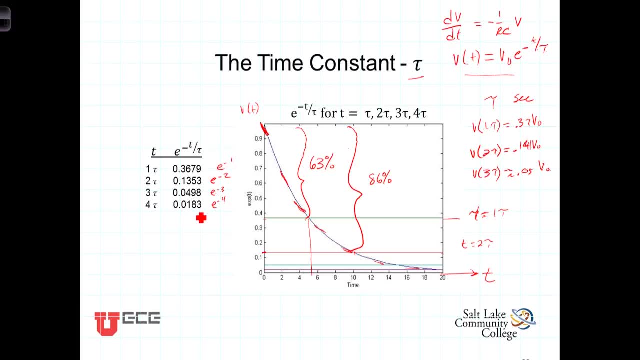 e to the minus 4 is approximately 0.02.. So the voltage across that capacitor after four time constants it has died out to about 2% of its original value, or we've gone 98% to our new value. 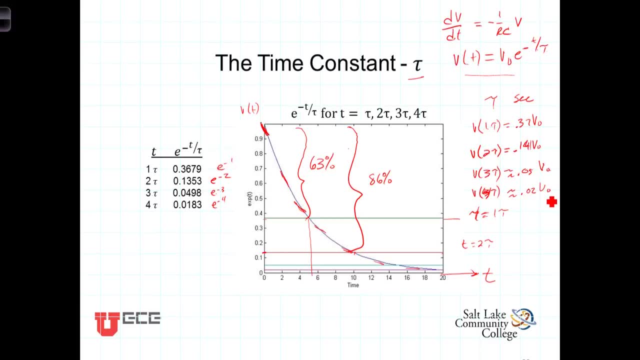 When talking about the rate of response of a circuit, we frequently will talk in terms of tau. Well, within two time constants, within four time constants. Of course, the time constant depends upon the circuit. Tau we have seen for an RC circuit.